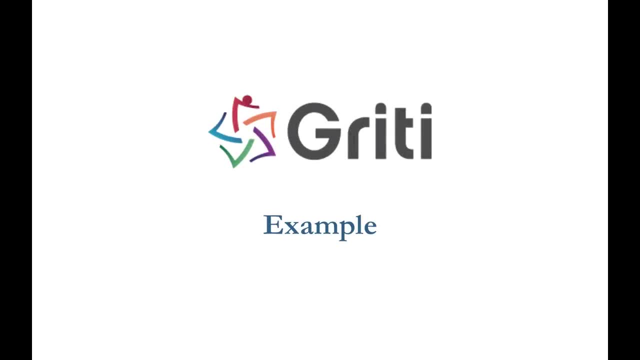 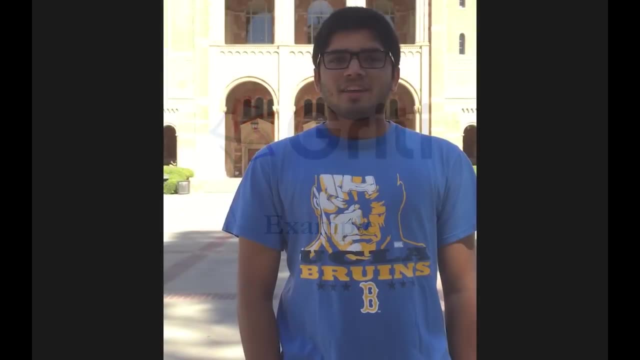 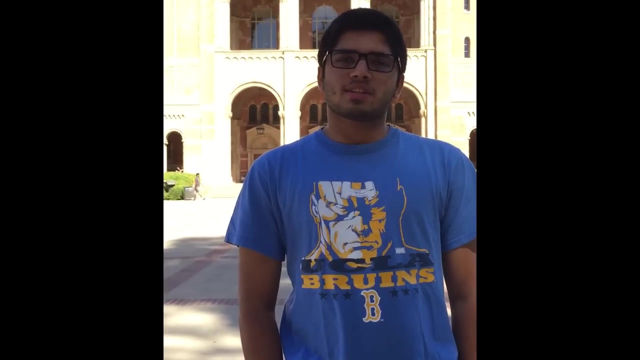 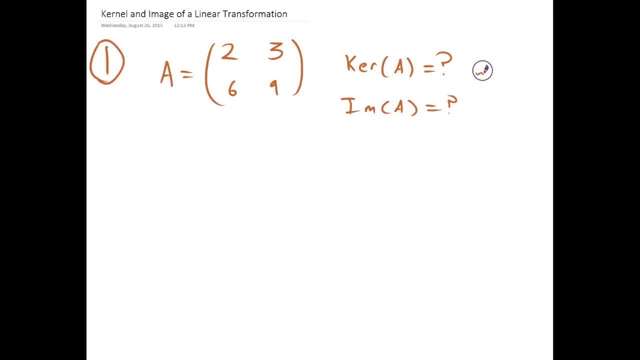 Hi, my name is Anil Nair and I'm an aerospace engineering student here at UCLA, and I'm going to help you by going over some math concepts and examples. Good luck. We're going to do some examples for the kernel and image of a linear transformation, So for 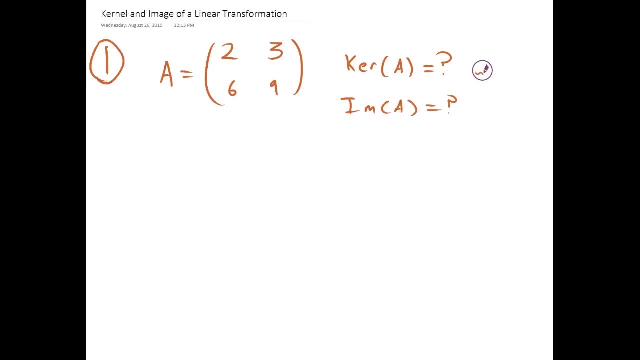 our first example: we have a matrix A, 2,, 3,, 6,, 9, and we're asked to find the kernel and the image of A. The kernel is the set of all vectors that the linear transformation defined by this matrix maps to 0. So the kernel is any vector x that maps to 0. 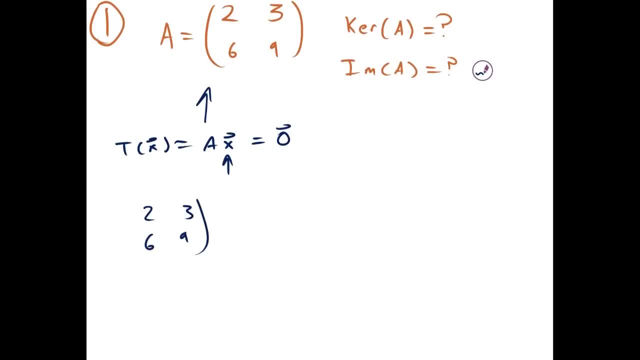 The way we find the kernel is: we look for all x and y for which this holds. And the way we solve this is by row reduction And we divide R1 by 2.. And we can subtract from R2, 6 of R1.. And we get 1,, 3 halves 0, and 0, 0, 0.. 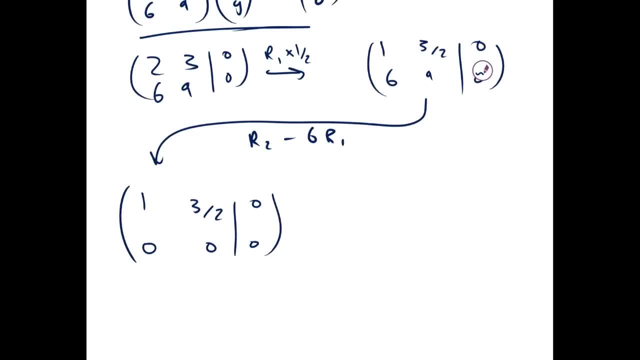 So this tells us that if x plus 3 halves y equals 0, then the vector is in the kernel. So x equals 3 halves y, y equals y. We can parametrize this. Let's say that x- y has to equal 3 halves times 1 y. 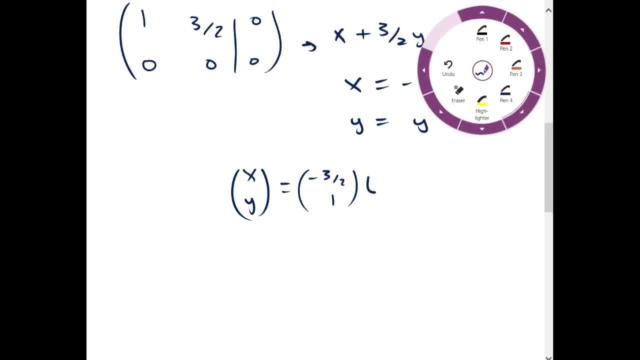 We can also just say: t is our parameter. t goes from infinity to negative infinity. This is the same thing as saying that the kernel- and this is the kernel of A, the kernel of A equals the span of this vector here, because it's all scalar multiples of that. 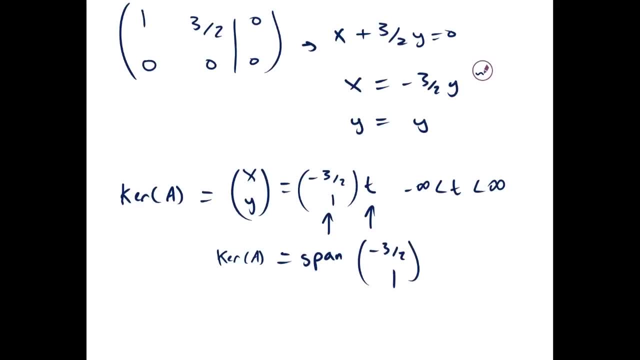 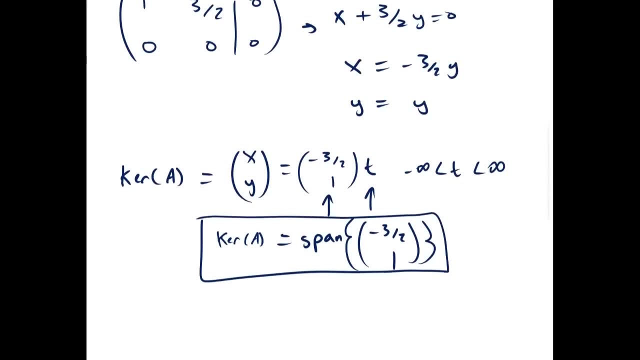 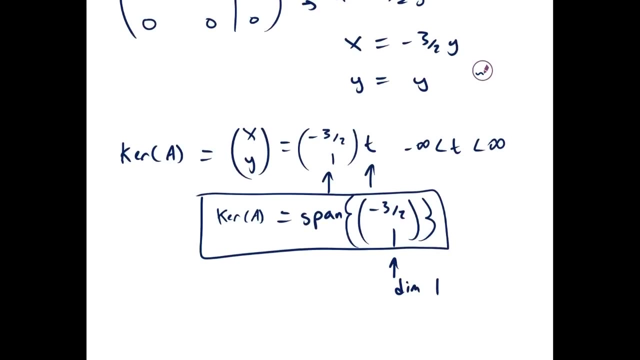 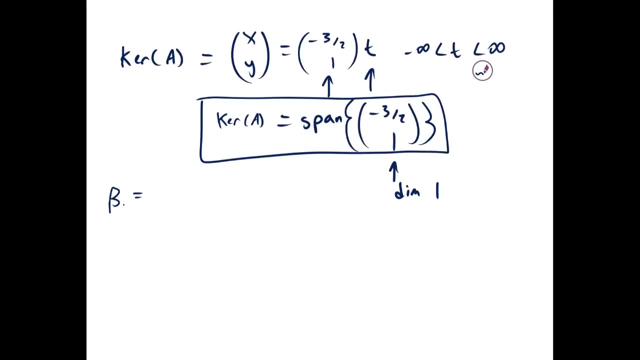 vector, So span of negative 3 halves 1.. So that's the kernel. So there's our kernel And it has dimension 1.. And if we wanted a basis for our kernel, let's say beta is the basis for the kernel, beta. 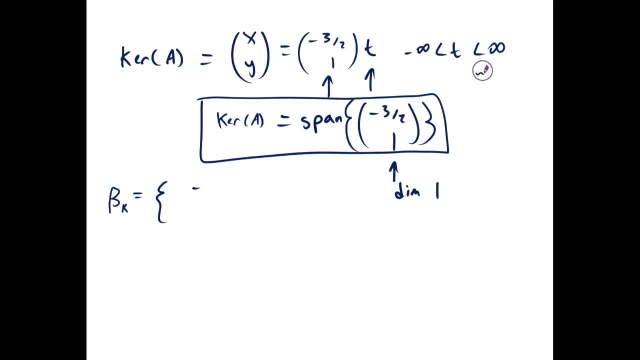 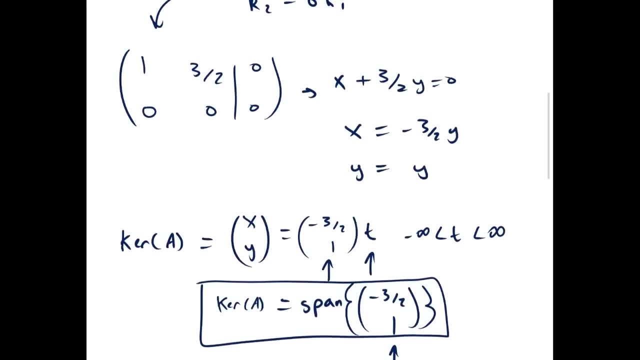 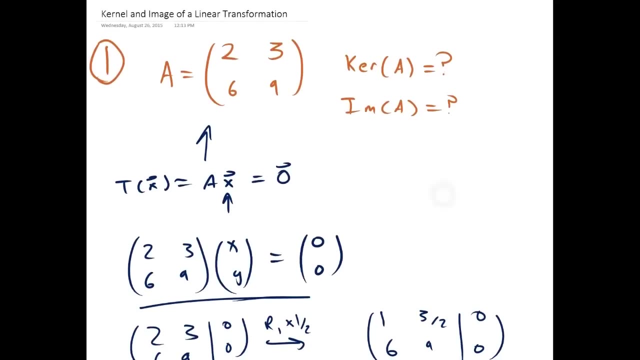 sub k, that basis would just be negative. 3 halves 1.. Okay, And by the rank nullity theorem, if you haven't watched that video yet, that's okay. we know that, since the dimension of the kernel is 1, and the dimension of the target space is. 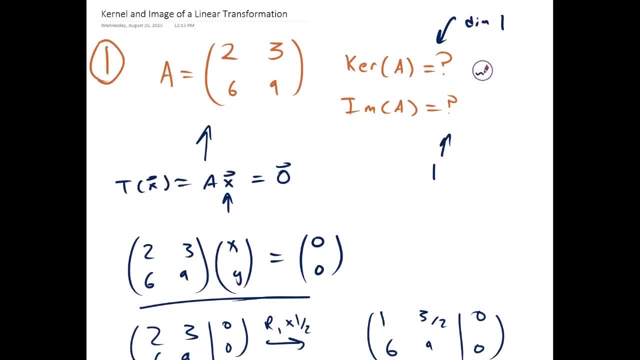 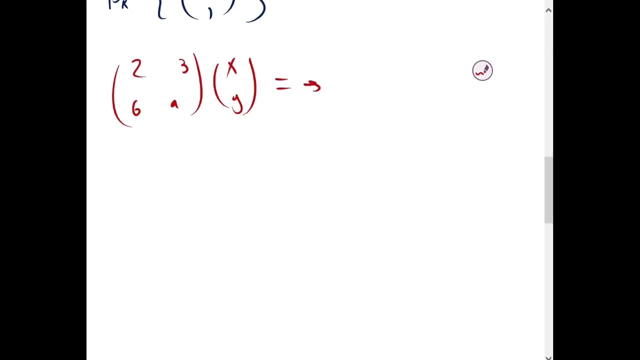 2, because we have a 2 by 2 matrix, the image should have also dimension 1.. Let's go ahead and find the image. The image is the set of vectors that the linear transformation maps to, So it's this set right here, whatever this equals. 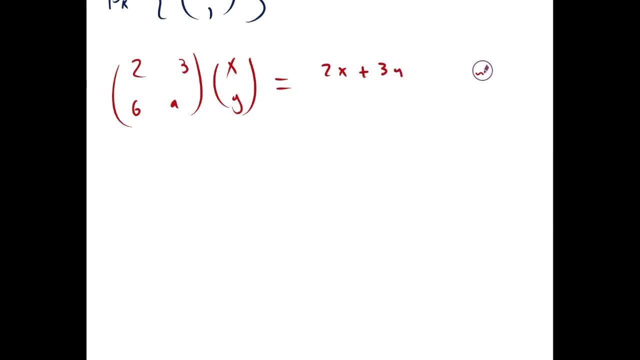 So that's going to be 2x plus 3y and 6x plus 9y. Okay, We can also write it like this: x times the column vector 2, 6, and y times the column vector 3, 9.. 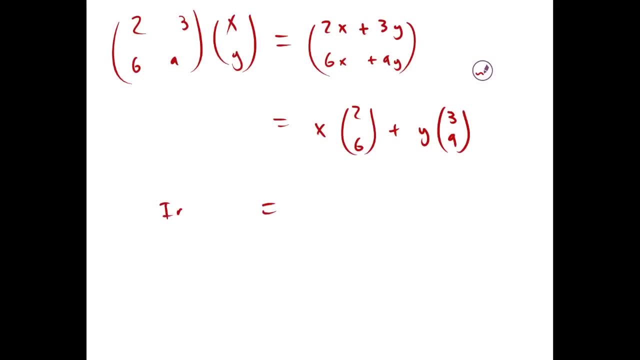 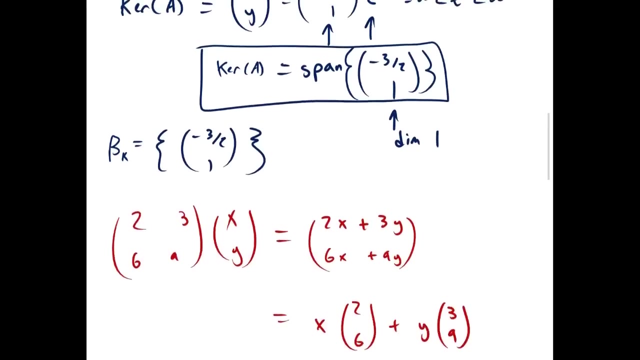 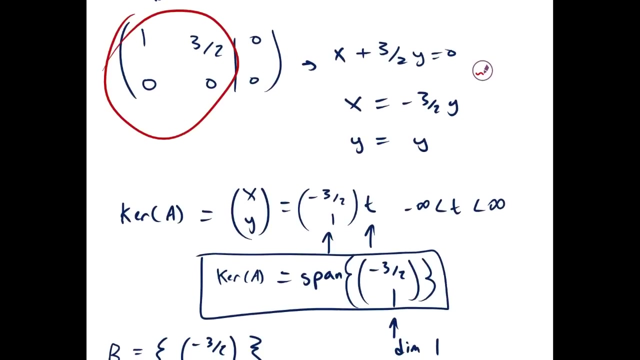 And that means that the image of A equals the span of these vectors. Okay, Okay, But actually one of these vectors is redundant. This is just a multiple of the other, And you can tell that's the case because when we found the reduced row, echelon form. 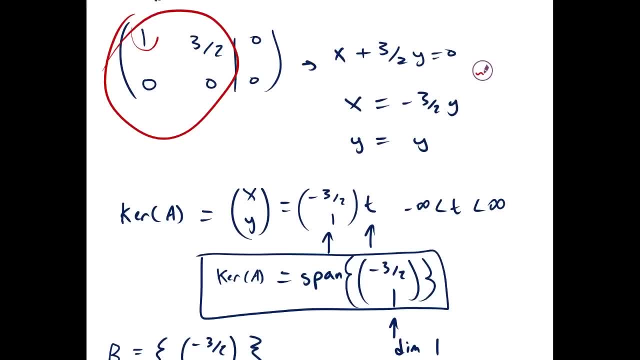 of that matrix we got only one leading one, So that means the second column is redundant. Specifically, it is 3 halves times the first column. We took the first column and we took the second column. We took 2,, 6, and multiplied it by 3 halves. we get 3, 9..